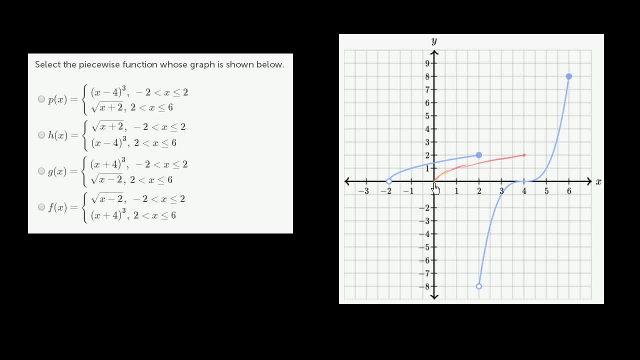 So square root of x looks like this And this just looks like square root of x. shifted 2 to the left, So this looks like square root of x plus 2.. This one right over here looks like square root of x plus 2.. 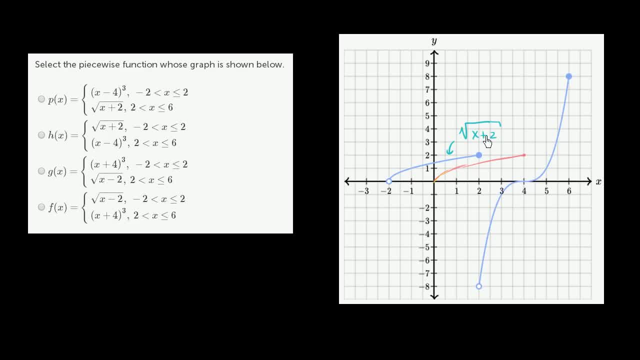 And you could verify that When x is negative 2, negative 2 plus 2, square root of that is going to be 0.. And it's not defined there, But we see that if we were to continue it would have been defined there. 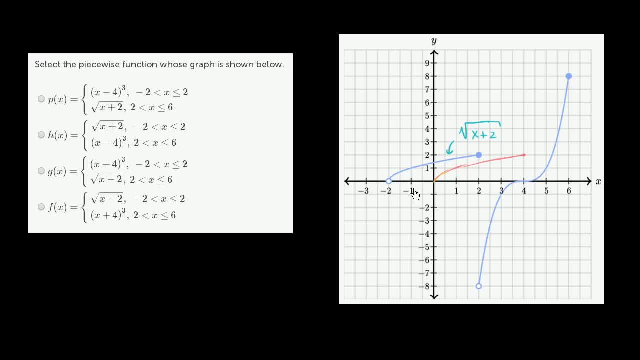 But let's try some other points. When x is negative, 1, negative, 1 plus 2 is 1.. Principal root of 1 is 1.. Let's try 2.. When x is equal to 2, 2 plus 2 is 4.. 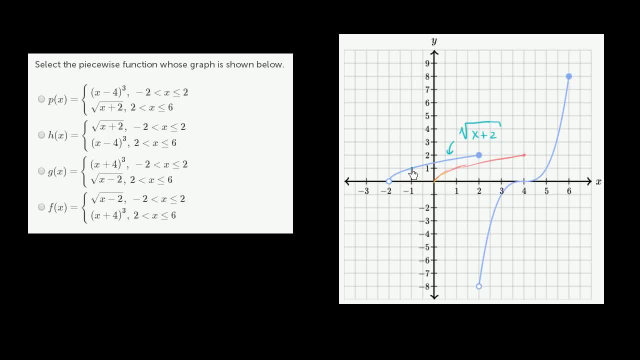 Principal root of 4 is positive 2.. So this looks like a pretty good candidate. So it looks like our function would be- and I'm not going to call it anything, because it could be ph, g or f, But this function if I were to write it out. 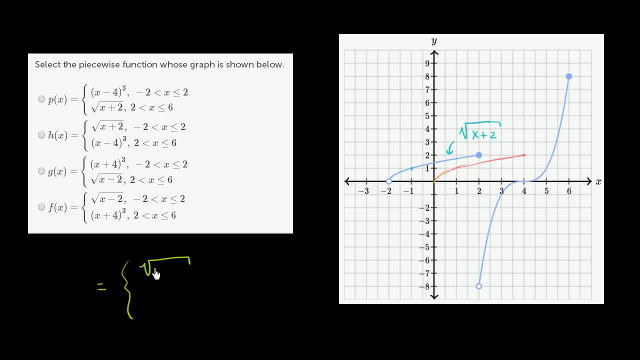 it looks like over this first interval, so it looks like it's the square root of x plus 2. for negative 2 being less than x, It's not defined at negative 2.. But as long as x is greater than negative 2,. 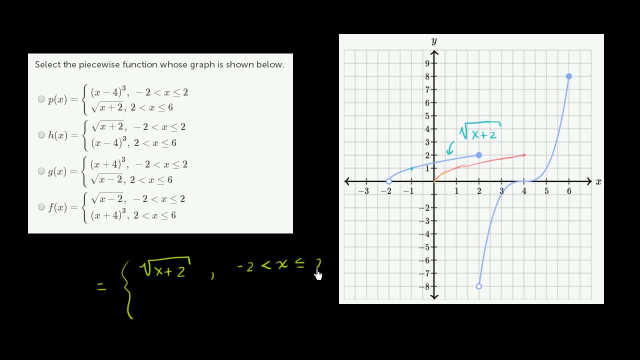 and x is less than or equal to 2.. So that's this part of the function, And then it jumps down And now this looks like a little bit more complicated. This looks like x to the third. x to the third looks something like this: 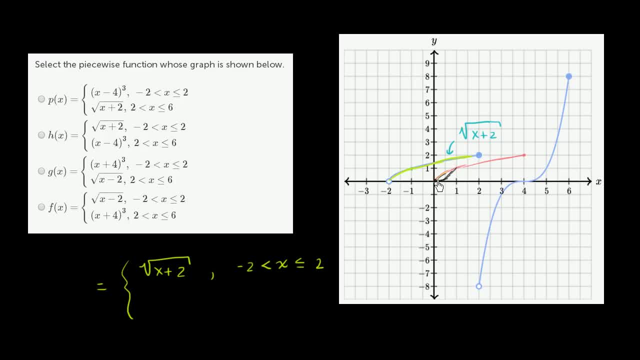 So x to the third power looks something like that. So let's see: negative 2 to the third power is negative 8.. So it looks something like that. That's what x to the third looks like. So 2 to the third power is 8.. 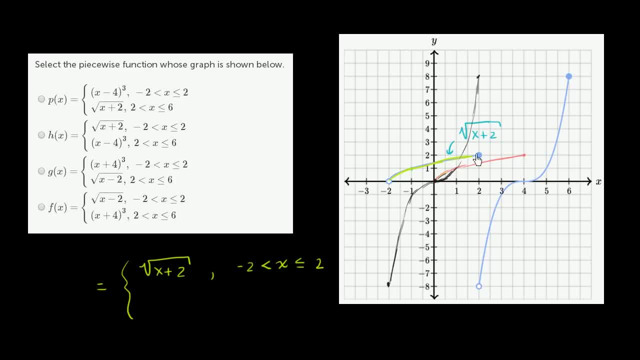 So x to the third looks something like that. This looks like x to the third shifted over 4.. So I'm guessing that this is x minus 4 to the third power. But we can verify that When x is equal to 4, 4 minus 4 to the third power.